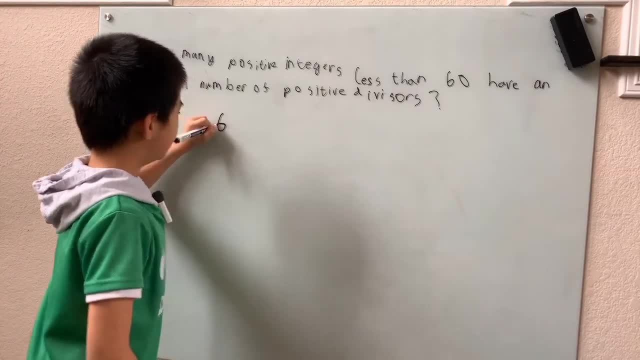 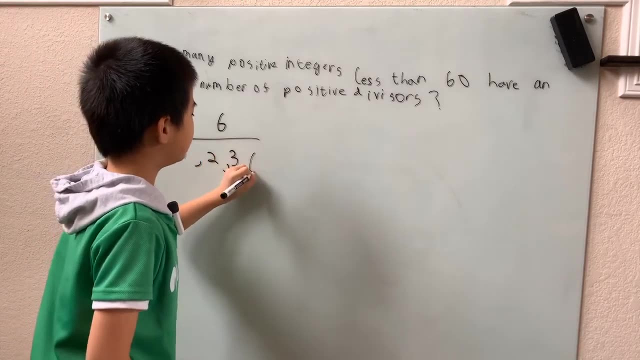 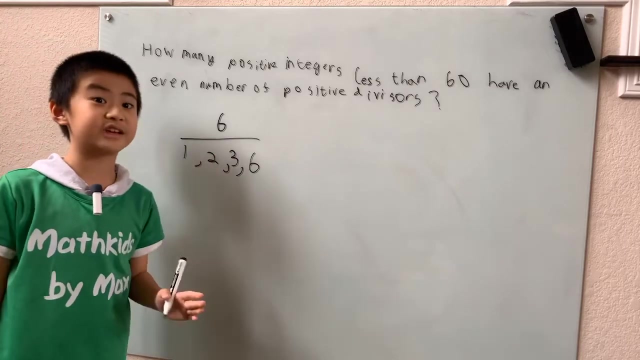 For example, if you want all the divisors of 6,, well, we know 6 is divisible by 1,, 2,, 3, and 6.. But we also know that 1,, 2,, 3, and 6 are all factors of 6.. 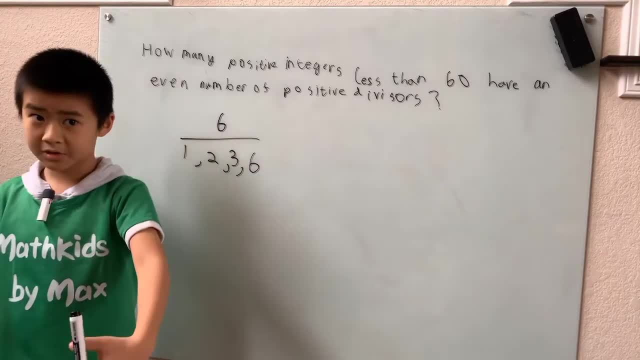 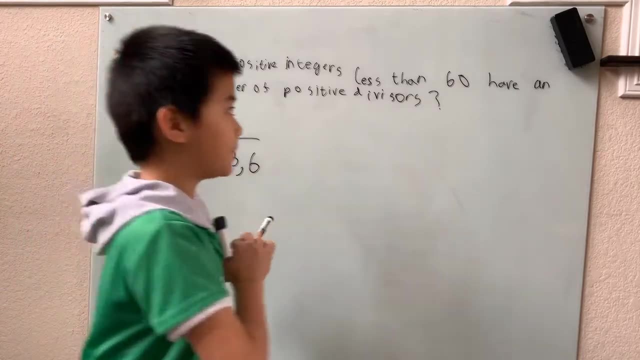 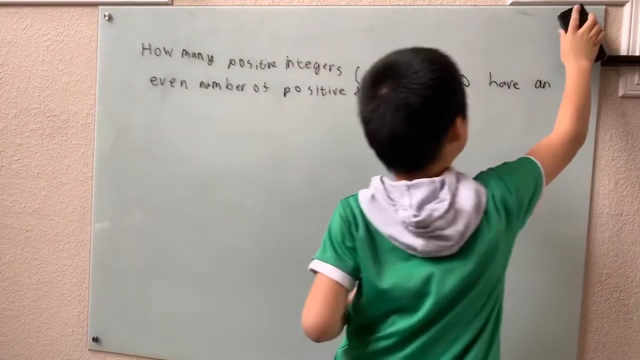 So for a number to be a divisor of another number, then it also has to be a factor of that same number. So we know that's true. So let me understand the not exactly very fancy part. What's a divisor? Let's play around with the problem a little bit. We're going to try some numbers. 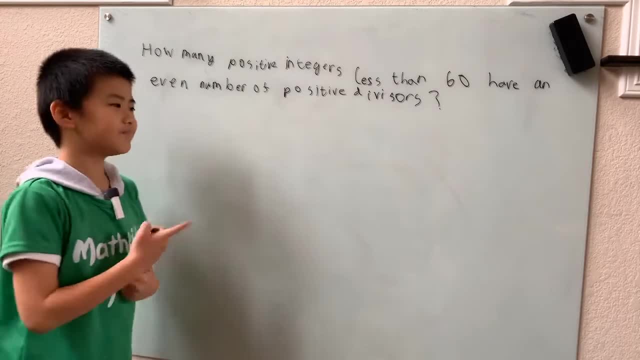 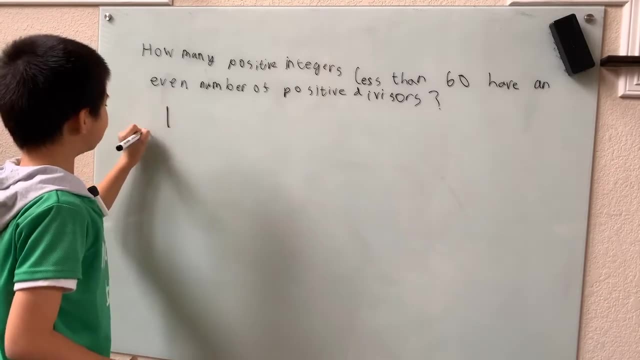 We're going to try to list all the factors. I mean, we're going to try to list the factors of all the numbers from 1 to 5.. We'll start with 1.. Well, 1 is pretty easy. That's just 1 times 1.. 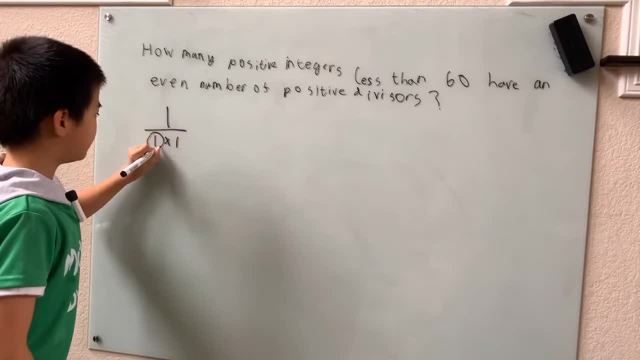 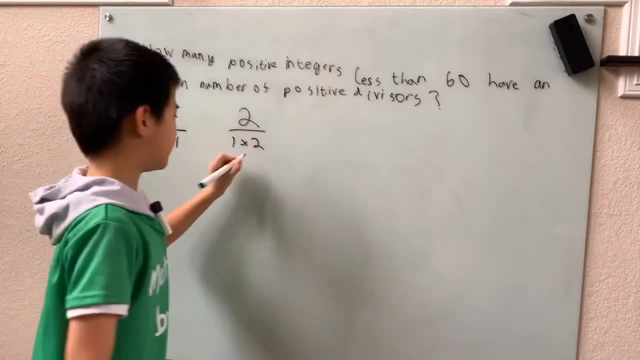 1, we have an odd number of factors. That's our only factor. Now we try 2.. Well, 2 is prime and we just have 1 times 2.. That's also pretty easy. Same: We have 1 and 2.. That's an even number of factors. 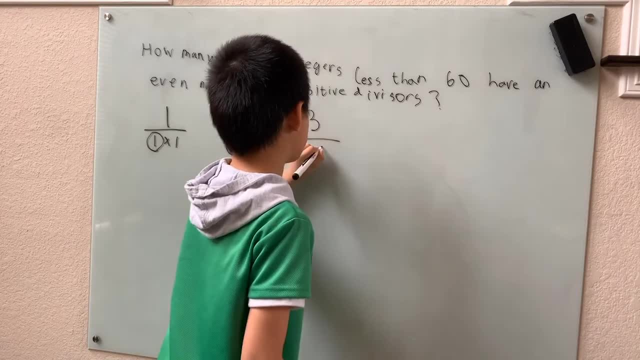 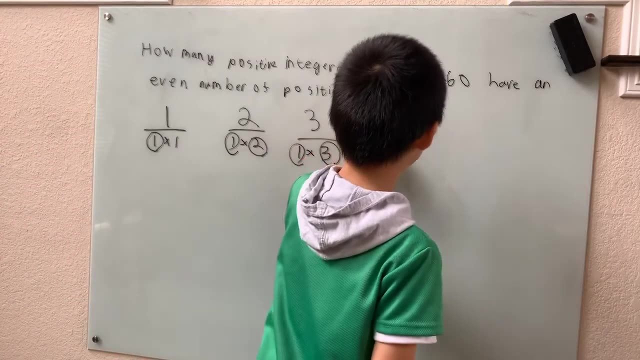 And 3 is not very interesting. We just have 1 and 3.. Even number of factors as well. But 4 is a little special because if I take a look at the factors of 4, I see 1 and 4 and 2 times 2. I see two pairs. 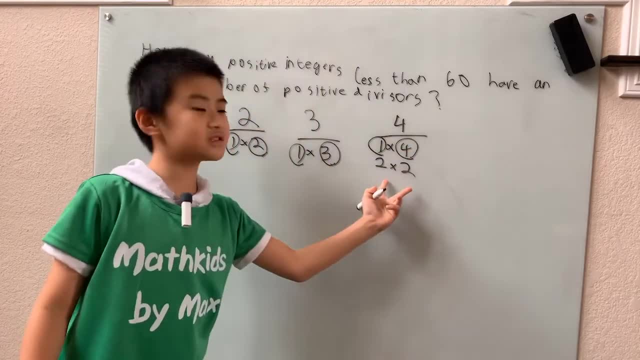 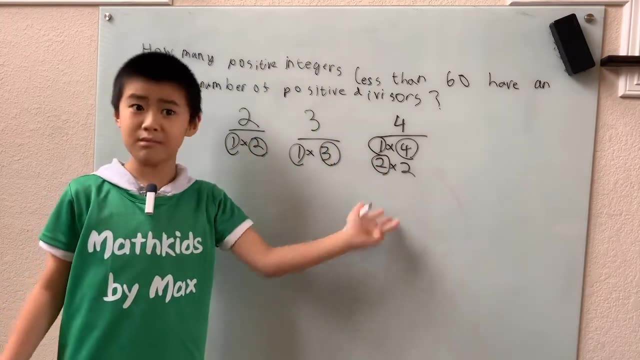 But when I circle 1 and 4, we don't want to circle both of these. Only one of these is a factor. I mean, I can't say both of these is a factor, because these are the same numbers. Now let's take a look at 5.. 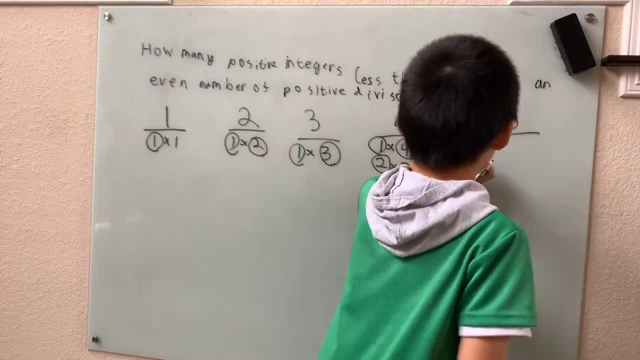 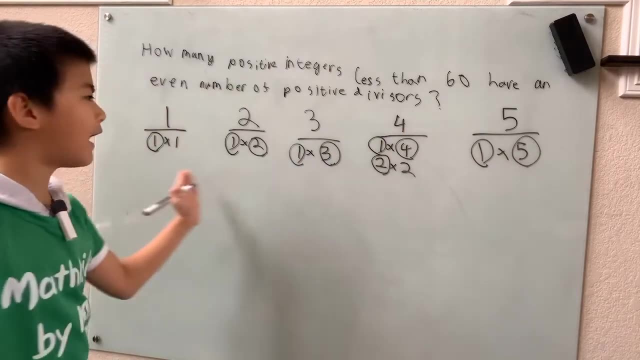 See if that has an even number of integers. I mean even number of factors Or odd. that is, 5 is also prime. It just has two factors. But look at what we have here. Numbers that have an odd number of factors are 1 and 4.. 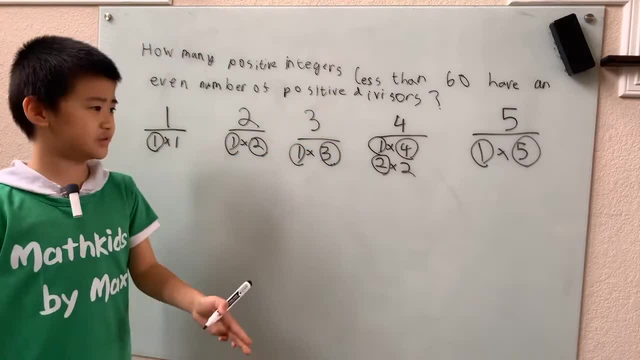 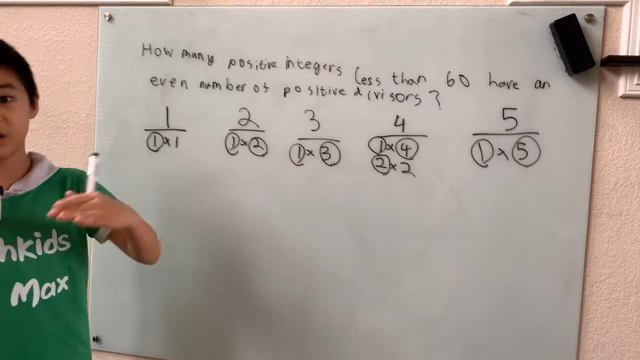 What's so special about 1 and 4? They're the perfect squares, But let's just work with all perfect squares. I mean, is it like all perfect squares have an odd number of factors and all the numbers that aren't perfect squares have an even number of factors? 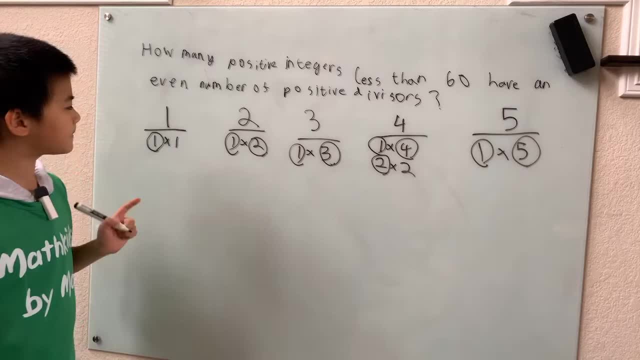 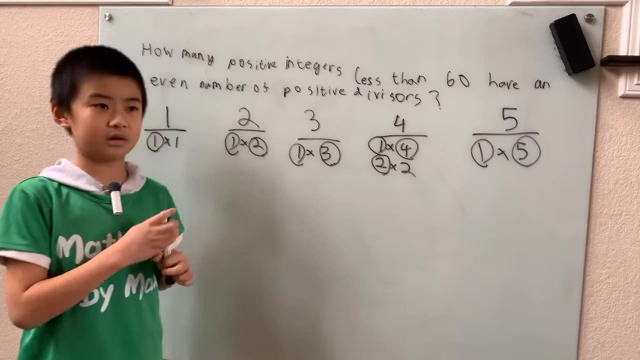 No Perfect squares have an even number of factors. Well, let's check that out. So let me think: If we have a number, well, the factors of that number, like a number, the factors of it is always something times something. 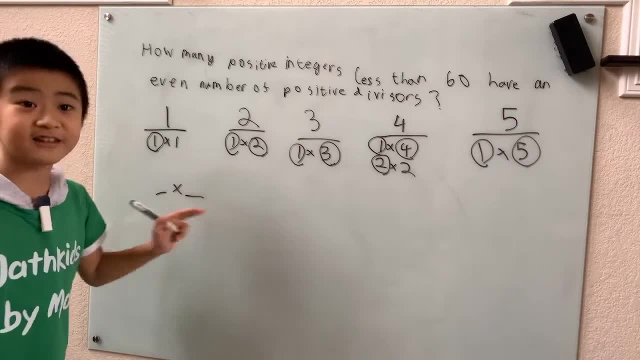 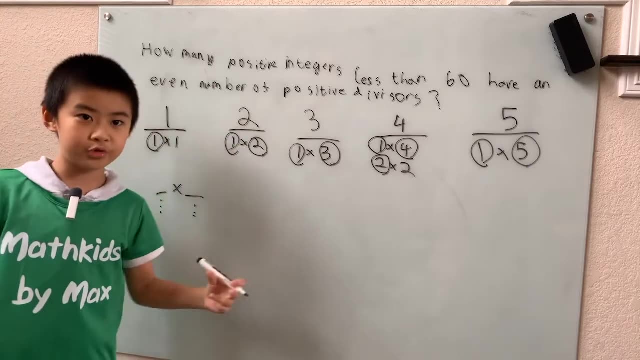 We can't have blank times, blank times. blank, It's not three numbers, It's just two. So we're going to keep going like this. They're just pairs 2, 2,, 2,, 2, 2.. 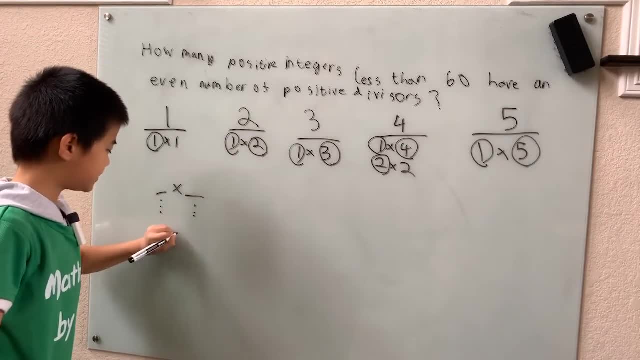 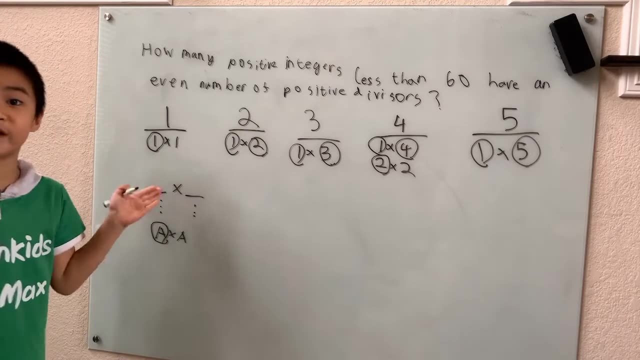 Until we get to a number. that's something like a times a. That's something like a times a. Well, a times a. only one of these is a factor of whatever number we're trying to find, Because we can't say: well, 2 and 2 is a factor of 4.. 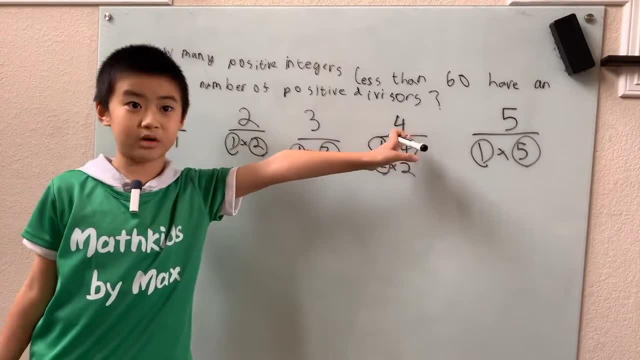 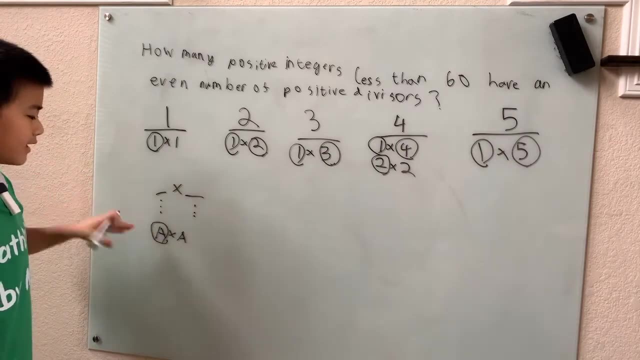 I mean, that's pretty confusing. Only 2 is a factor of 4.. We should say 2 is a factor of 4 instead of 2 and 2 is a factor of 4.. So now we know any number. that's not a perfect square. 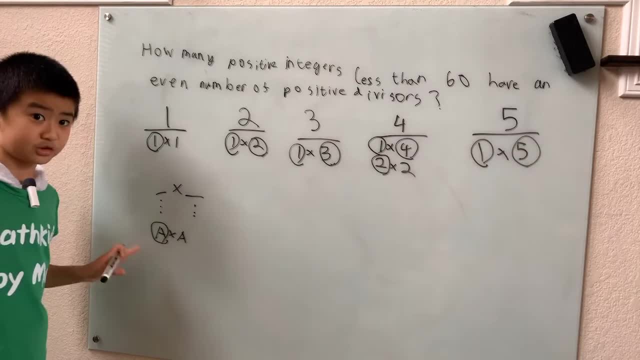 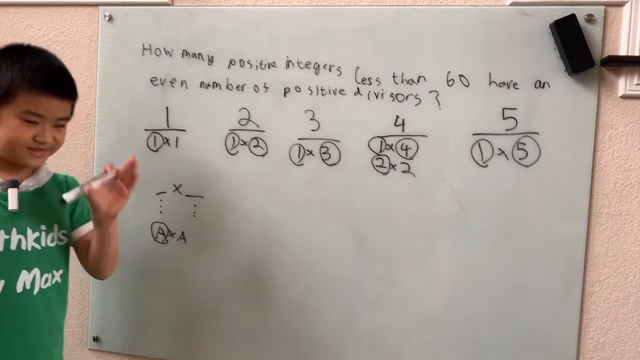 isn't going to have a times a in their factors list, So we're just going to have pairs, pairs, pairs, pairs. That's all it's going to have, Which means any number that doesn't have. I mean, that isn't a perfect square. 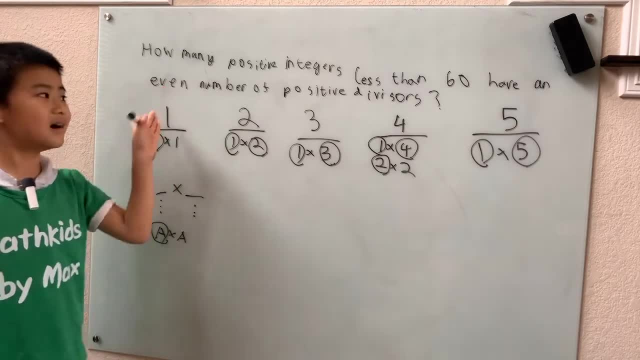 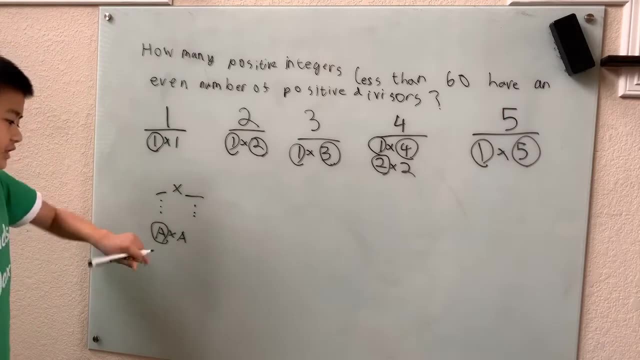 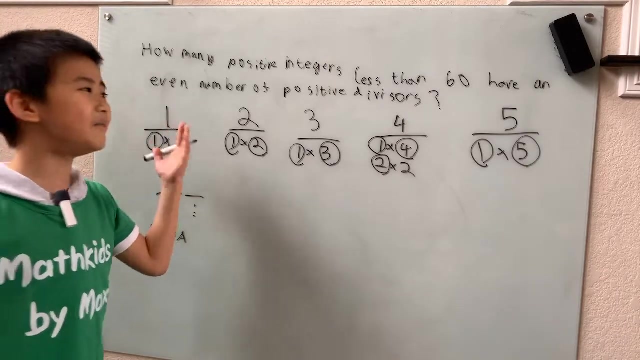 has an even number of divisors. But any number that is a perfect square has an odd number of divisors, Because it does have this a times a thing in it. So now we just have to count the number. we just have to count the number of perfect squares, from 1 to 60.. 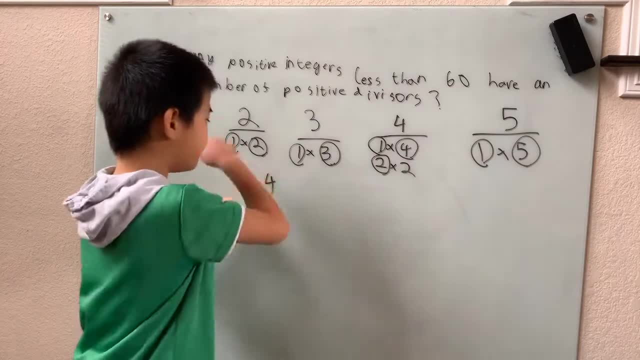 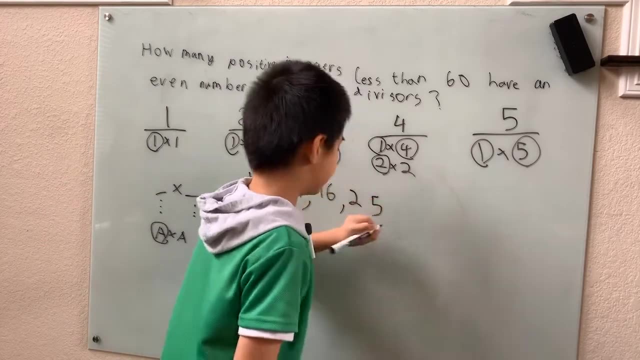 Well, that's pretty easy: 1 and 4,, 9,, 16.. All of these have an odd number of divisors: 25,, 36, and on and on and on 49.. Well, we're going to have 7 squared. 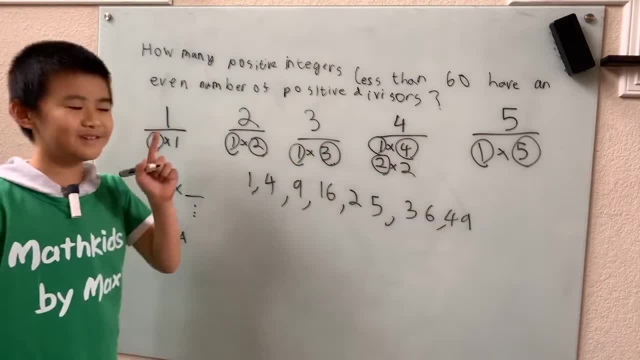 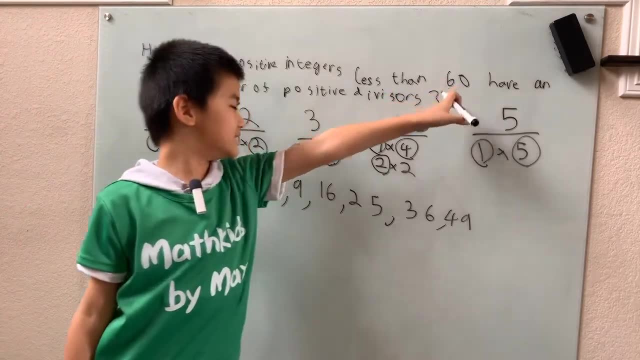 8 squared is 64. That's too large. But here's the thing. Don't be like you did all this work but then you get the answer wrong, The simple part. You don't want 60 minus our number.